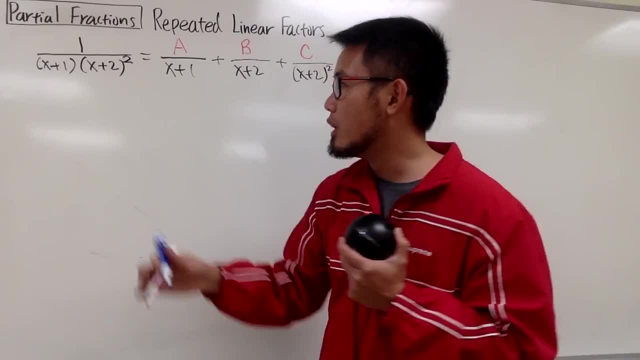 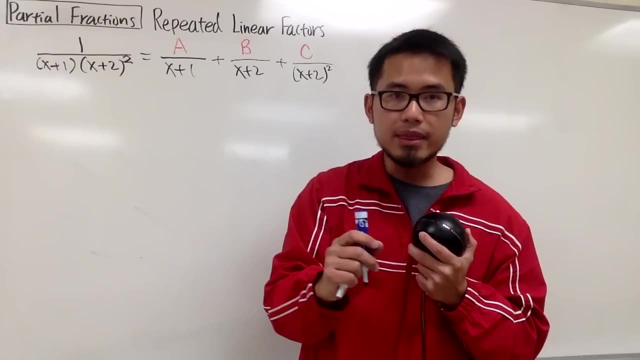 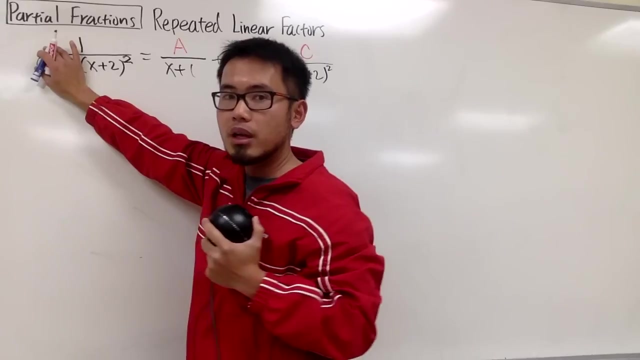 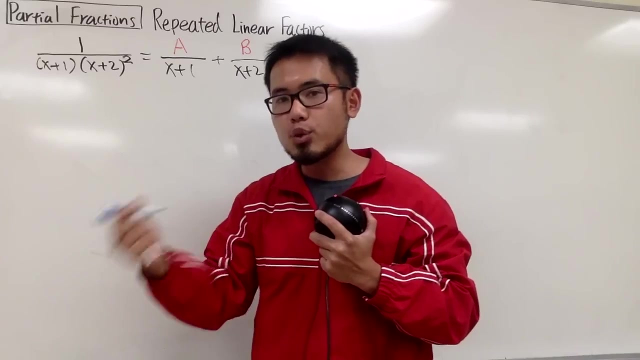 And you have to ask yourself: how can you make that factor equal to 0?? How can you make x plus 1 equal to 0?? Well, the answer to that is: let x equal to negative 1.. Well, once you cover this up, remember x is equal to negative 1, and plug in negative 1 into this x. now and work this out: 1 over negative, 1 plus 2 in the parentheses, and square Negative 1 plus 2 is 1, and the square of that is 1.. 1 over 1 is 1, so this right here is 1. Done. 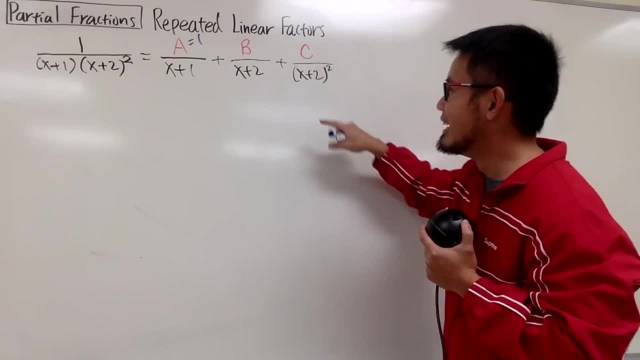 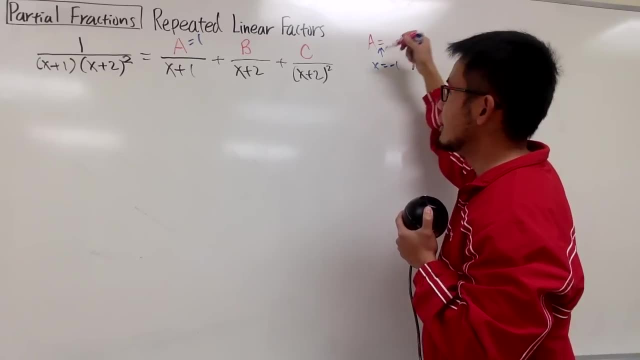 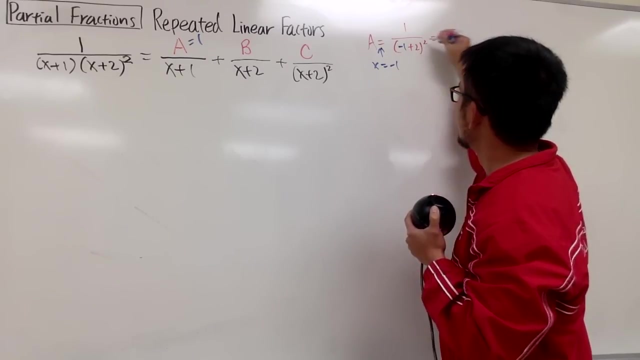 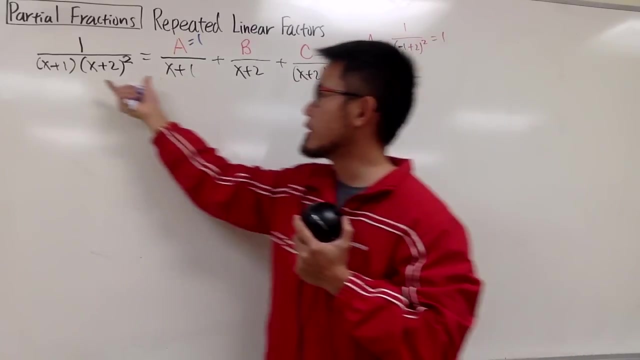 And in fact we can also do the same for c. right, And once again, a is just because we let x equal to negative 1, and then you see, this is 1 over negative 1 plus 2 square and you end up with 1.. Okay, We can do the same for c, because this right here has the same denominator. right here I get to cover this up from the original, because this and that are the same, Alright. 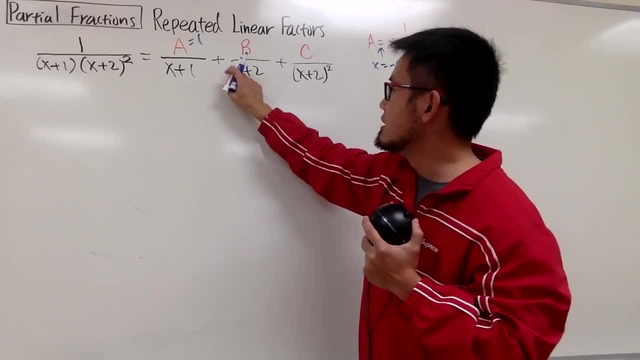 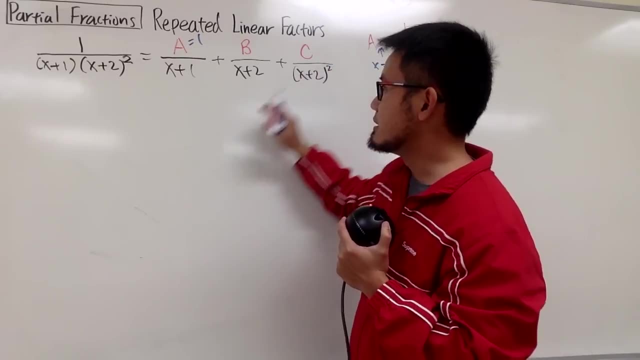 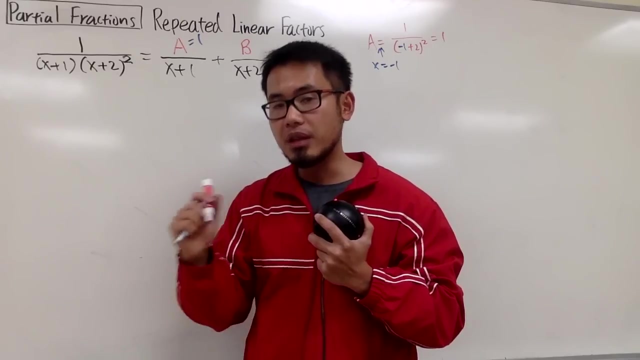 I cannot do the cover up with b, because this is x plus 2.. It's not exactly the same as 1 second of that. Okay. Anyway, to get c, I will cover this up And remember how can we make this factor equal to 0? I will have to let x equal to negative 2.. So I'll just put this down: c is equal to the situation where you let x equal to negative 2.. 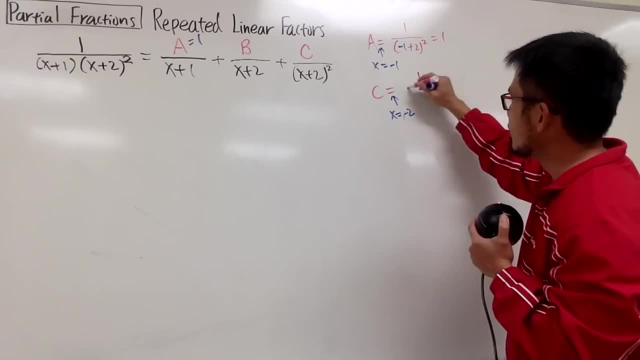 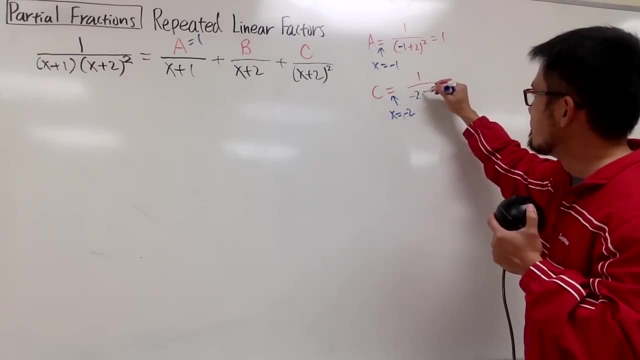 So in this case I will work this out for you guys. It will be 1 over. plug in negative 2 into the remaining part, namely just that Negative 2 plus 1, which is 1 over negative 1, which is negative 1.. And we get a c value right away as well. 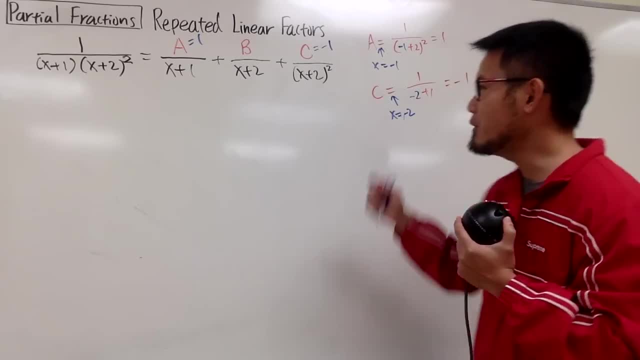 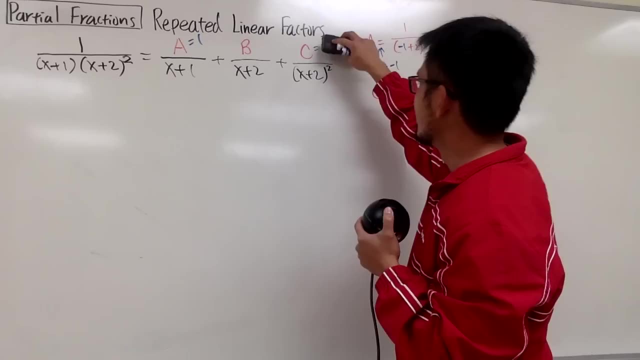 Okay, So this is the quick way to do cover up. It can also be in your head, because I did that in my head for a Okay, So keep that in mind, But remember this right here. Okay, Remember this right here. 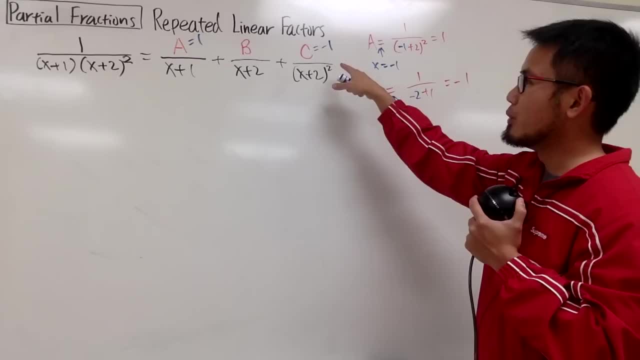 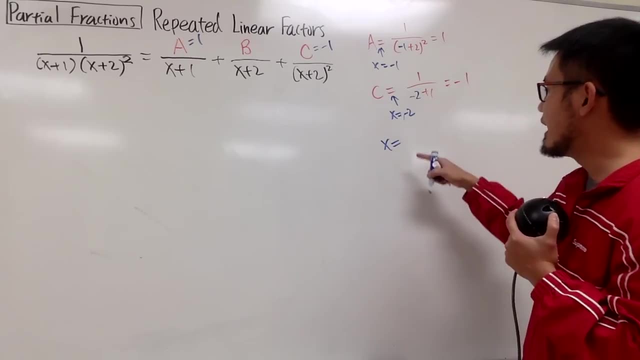 And once you have the a and c value, we can just say that x equal to another number that you haven't used yet. I can say that x is equal to 0, because this is easy And I can use this in the sense that I can plug in 0 into the number up here. 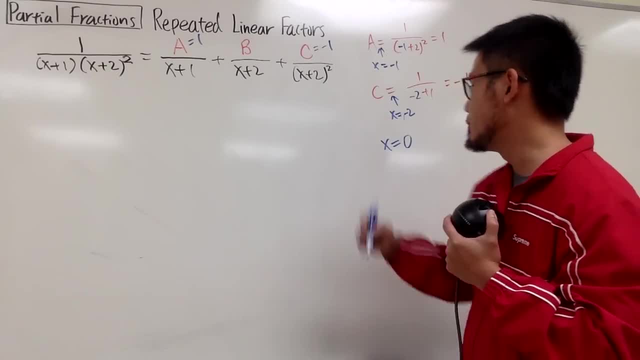 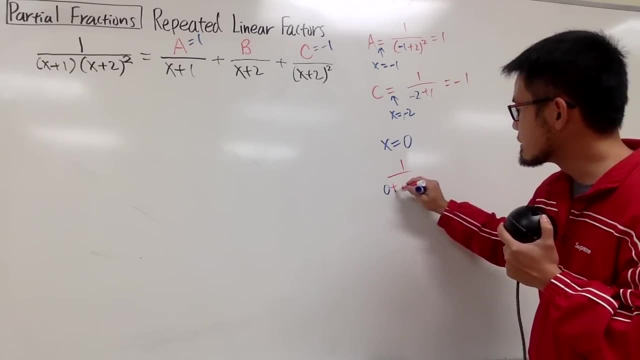 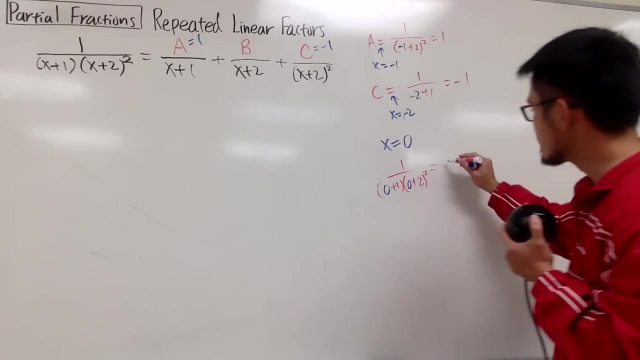 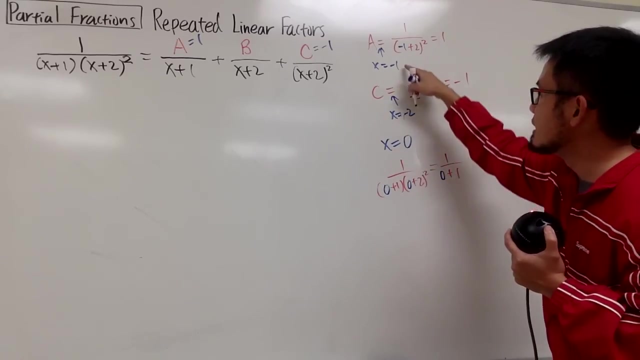 all the x and then I can find out the b-value. Let me do that for you guys real quick. So 1 over 0 into the x, so it's 0 plus 1 times 0 plus 2 squared, and make that equal to 1 over 0 plus 1.. I'm letting all the x equal to 0.. You can let x equal to whatever you want, besides negative 1 and besides negative 2, because you used it already And of course you should pick an easy number. 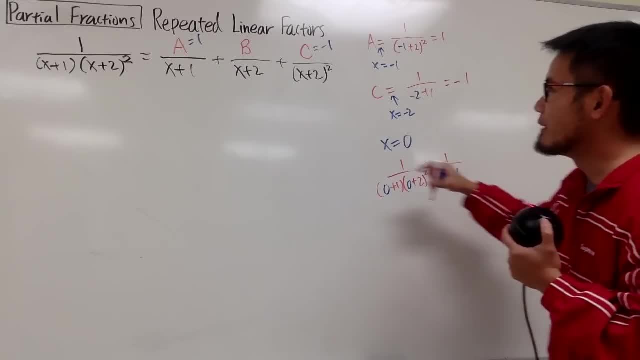 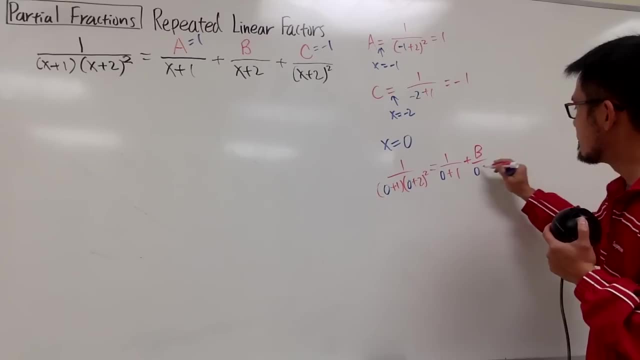 Otherwise it's going to be crazy. Anyway, plugging 0 into this x, we get plus b- I don't know yet right- And then 0 plus 2, and then plus c is negative 1 over. plugging 0 into here, we have 0 plus 2 squared. 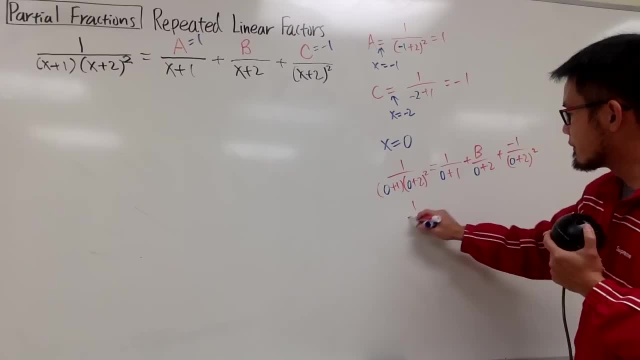 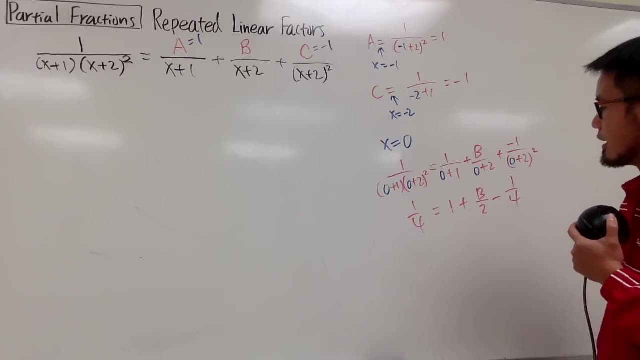 And you can work this out real quick. This is going to give you 1 over 4,. this is 1 plus b over 2, and this is minus 1 over 4, right And seriously. you can do whatever you would like. You can. this is 1 over 4, equal to this, and that is 3 over 4.. 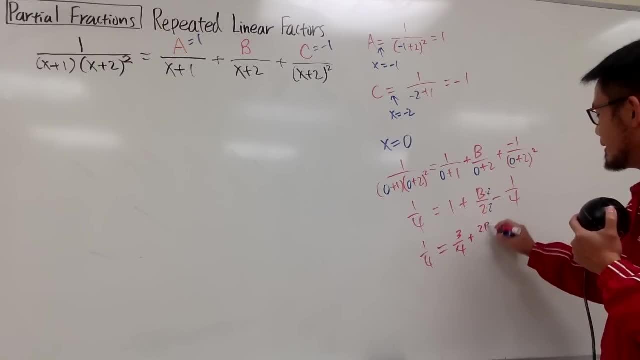 And you can get the common denominator which is plus 2b over 4.. And by now you should see b should be negative 1, because 2 times negative 1 is negative 2, plus 3 is 1, so that 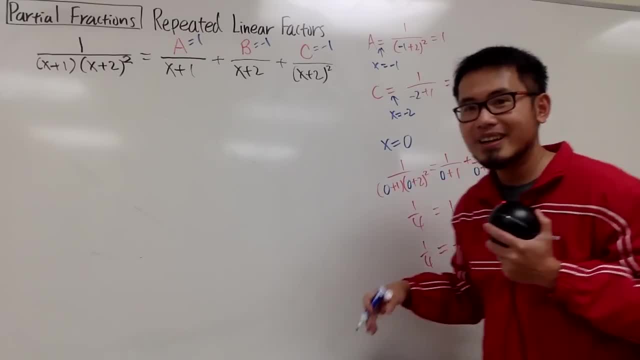 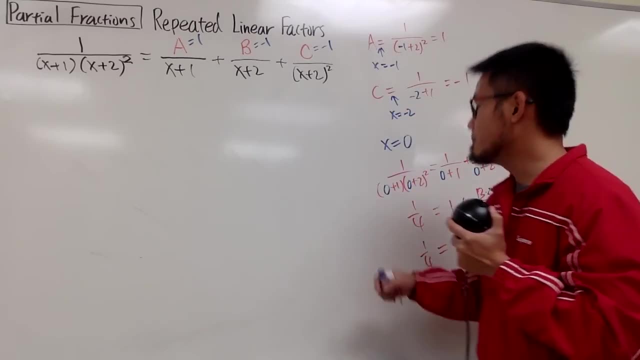 So we get it. b is equal to negative 1.. This is how the partial fractions work. This is how it's covered up as a work right. This is the quickest way. Well, I will explain why this works. This is how. 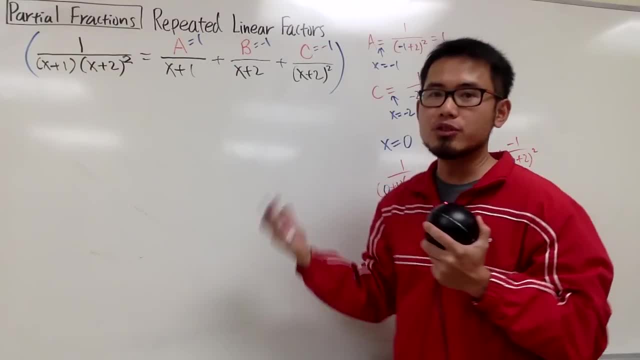 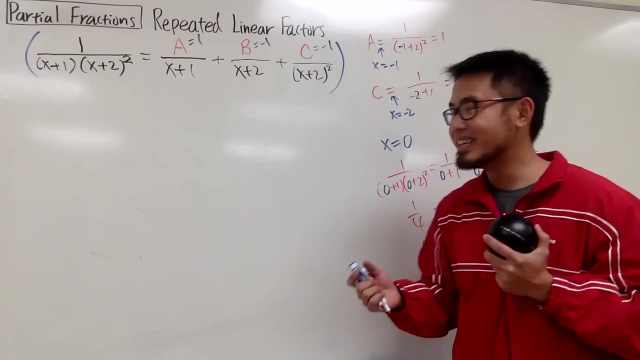 Usually you don't want to deal with an equation with a bunch of fractions, so what we can do is just multiply everything by the lowest common denominator. But that's kind of bizarre. If you have linear factors, do the following: yeah. 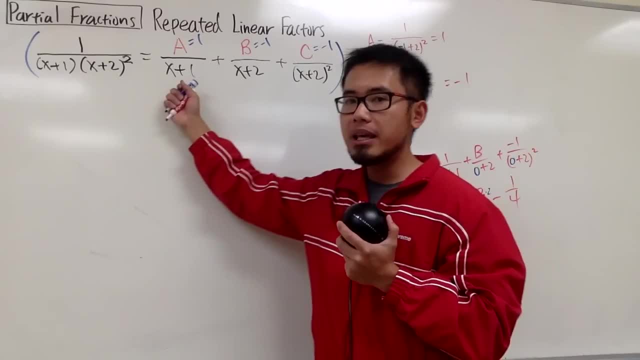 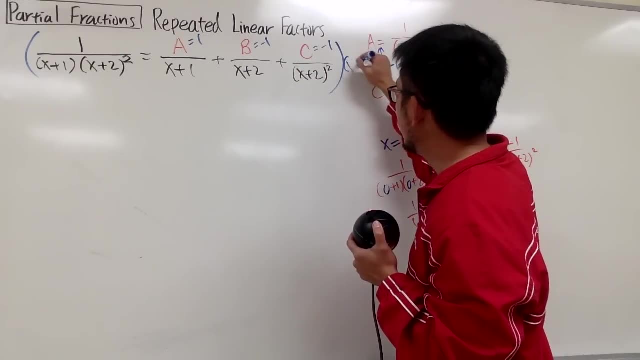 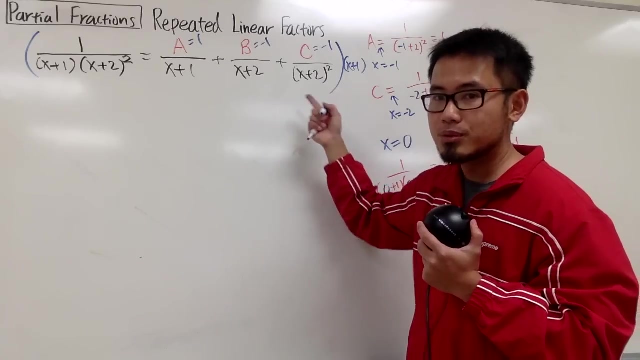 Suppose I want to figure out what a is, You can just do the following: Look at the denominator, which is just x plus 1.. I will multiply everything by x plus 1, only okay. And of course, take this: distribute, distribute, distribute, right. 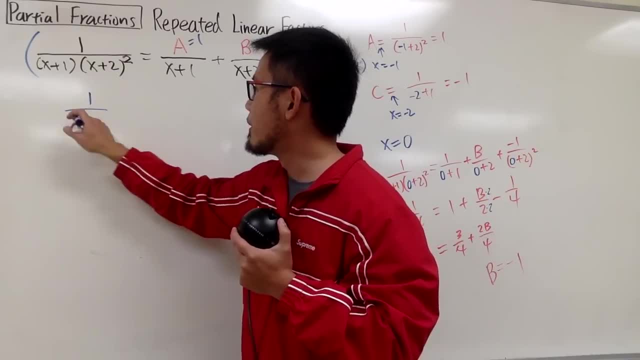 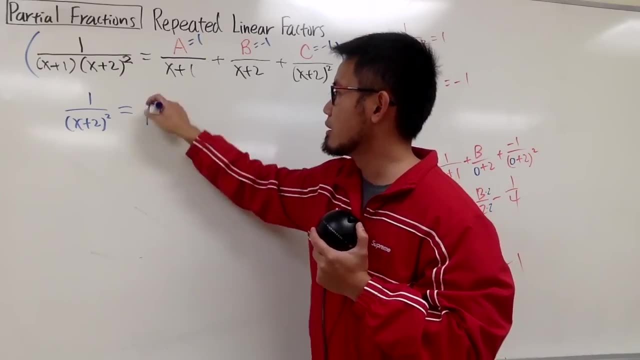 x plus 1 times. this guy is just 1 over x plus 2 squared And then x plus 1 times. this is just a. okay, I'm explaining why the cover-up method works. I know He's 1 already, okay. 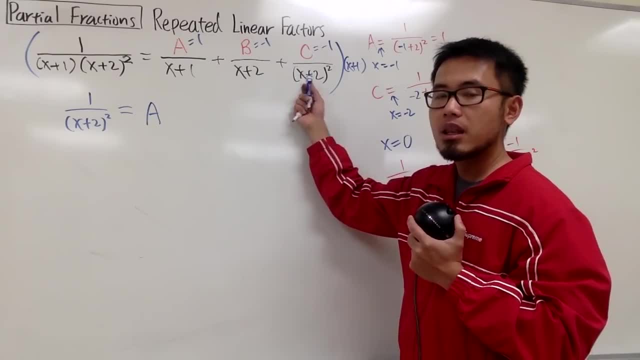 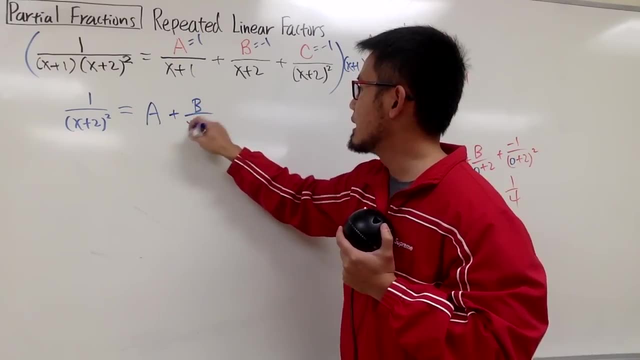 But anyway, check this out: When I take this, multiply this, and that nothing cancels out, I will still have the x plus 1, isn't it? So let me just put down plus b over x plus 2 times x plus 1.. 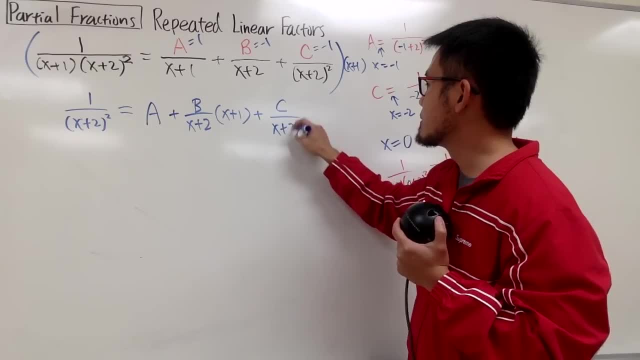 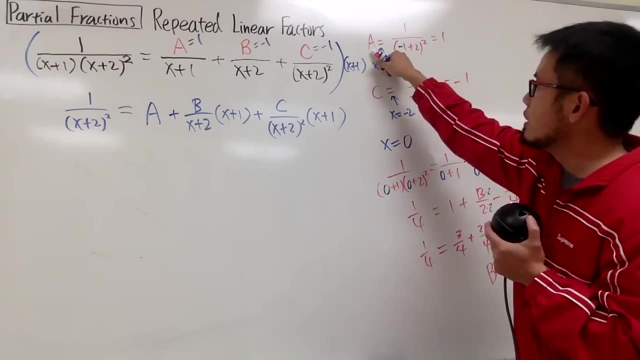 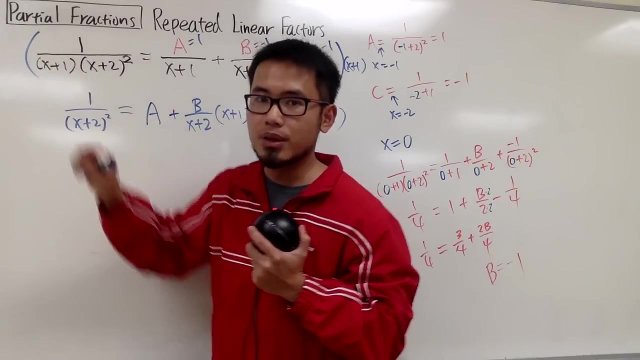 And then plus c over x plus 2, squared times x plus 1.. And remember earlier when we found a, we let x is equal to negative 1.. Because I asked you guys, how can we make this factor equal to 0?? 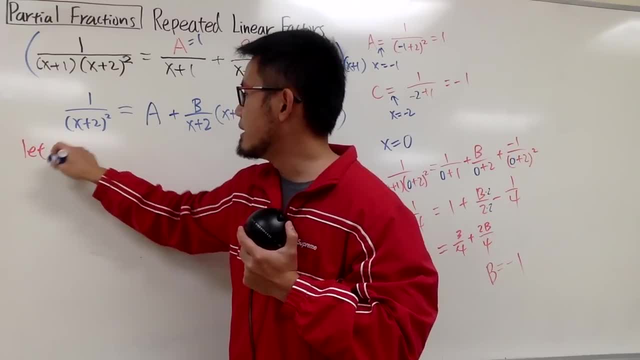 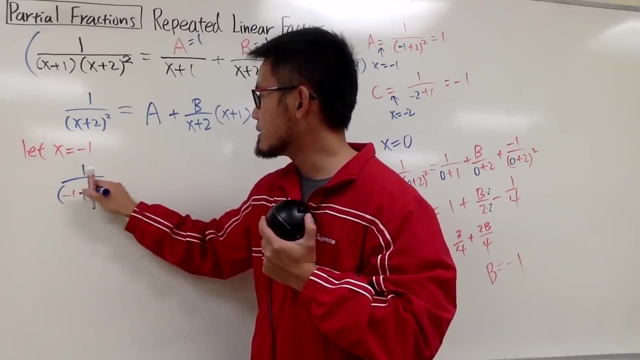 Now you see, by letting- I will just put this down By letting- x equal to negative 1.. Well, I will just do 1 over negative, 1 plus 2 squared, And the a is right here, And check this out. 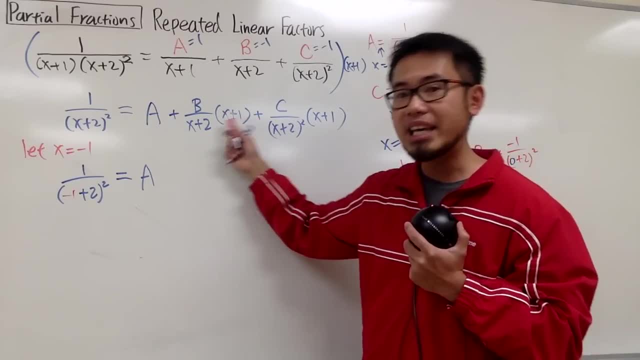 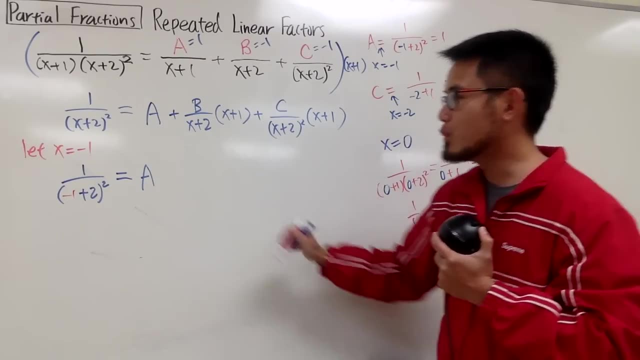 When I plug in negative 1 to here: negative 1 plus 1 is 0. That kills this term. Plug in negative 1 into here: negative 1 plus 1 is 0. That kills this term. So we just have plus 0 plus 0.. 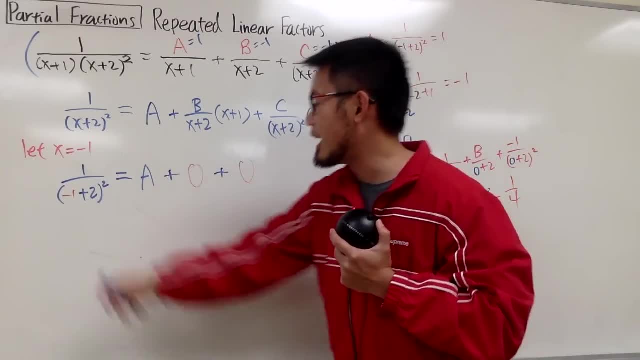 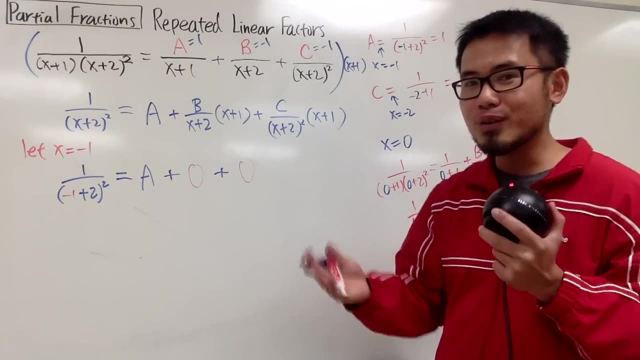 So the b and c- they don't matter And I just have a- is equal to that, And that's exactly what we did earlier, isn't it Okay? So you get a is equal to 1. And hopefully you guys see it. 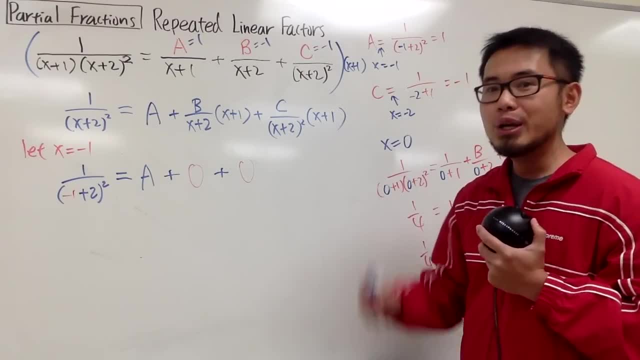 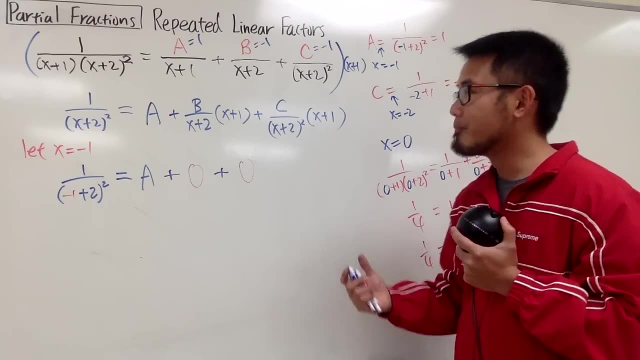 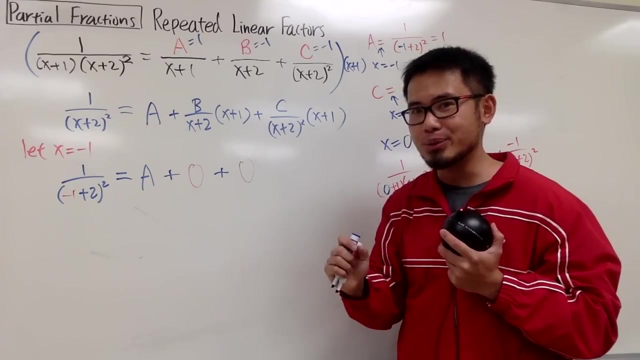 If you want to figure out what c is, what do you have to multiply? You multiply by the same exact denominator, namely x plus 2 squared, And when you do that, this term will have x plus 2 squared. This term will still have one more, x plus 2, right? 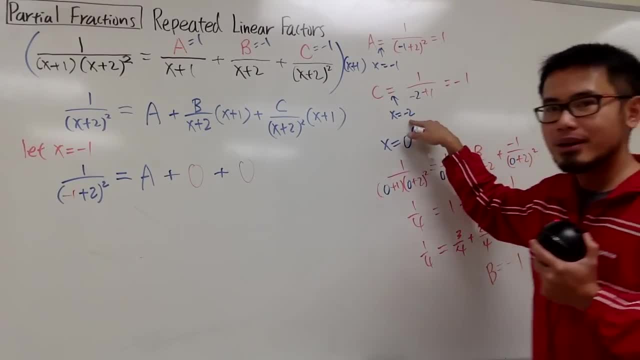 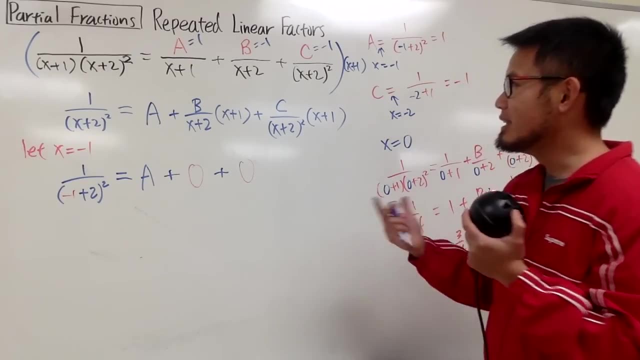 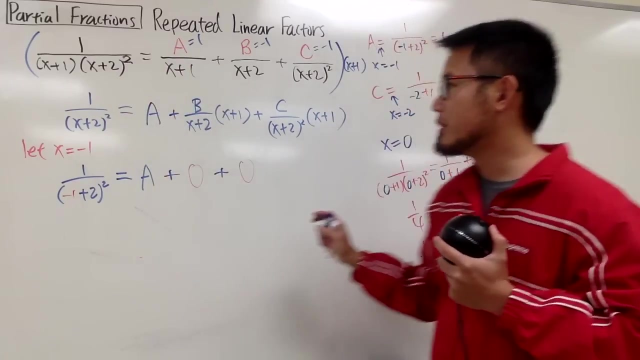 So when you let x equal to negative 2,, that will kill the b as well. Okay, So you should try that on your own And in the end you do see that. well, this is the quickest way to do it when we have linear factors in the denominator, like this: 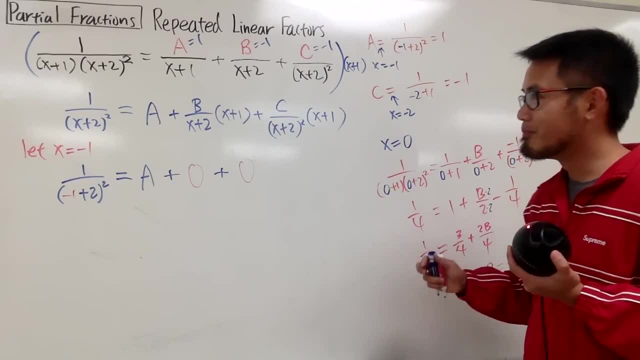 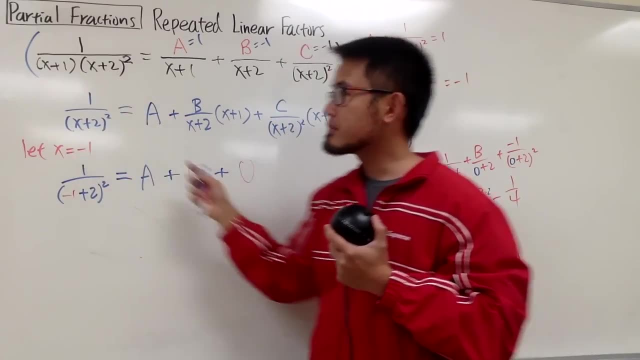 Okay, So it's like: yeah, Or, if you would like, you can just do the old-fashioned way: Multiply everything by the lowest common denominator And then collect terms and then match coefficients. If this requests, I will do that video for you guys.